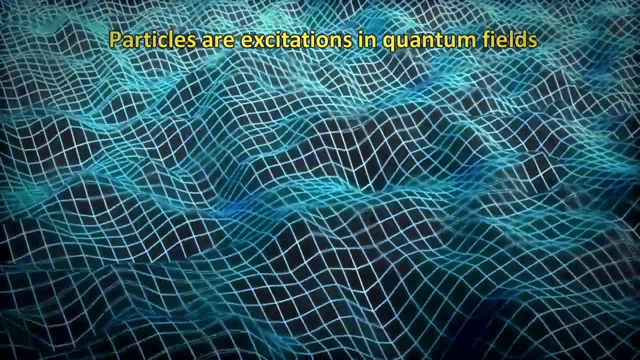 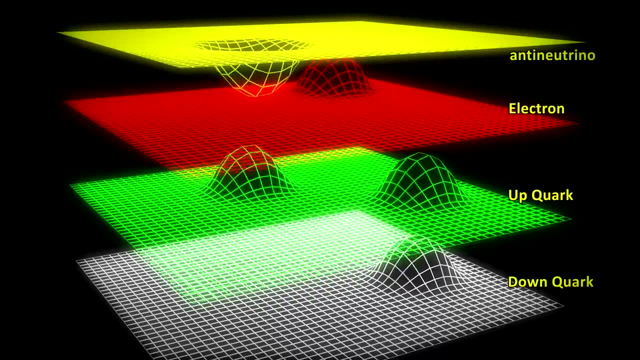 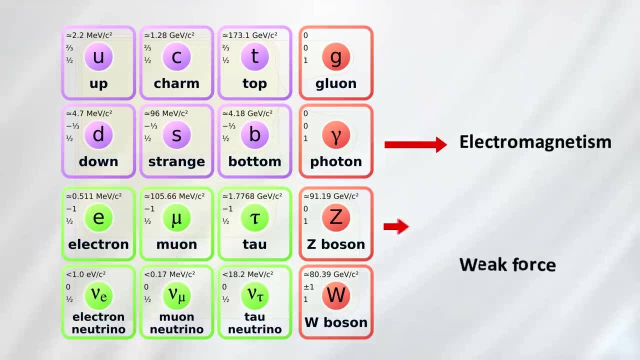 we can very accurately describe the other three forces in terms of quantum field theories. These theories explain how particles like quarks and electrons interact with each other via these three forces. Each force is mediated by a force carrier, also called a mediator. The electromagnetic force is mediated by the photon, the weak force by the W and Z bosons. 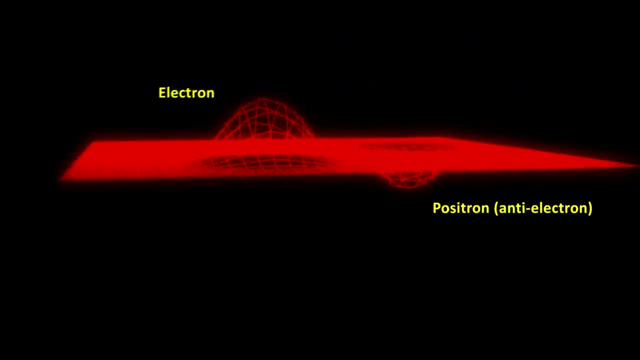 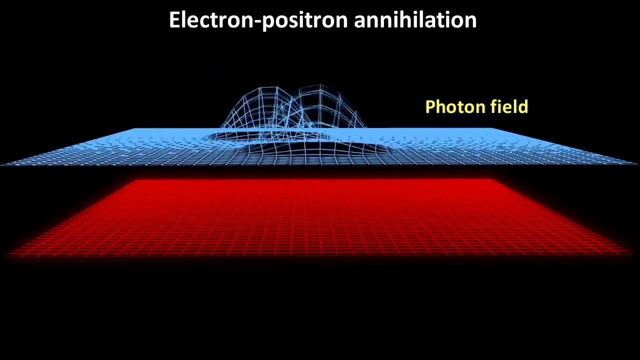 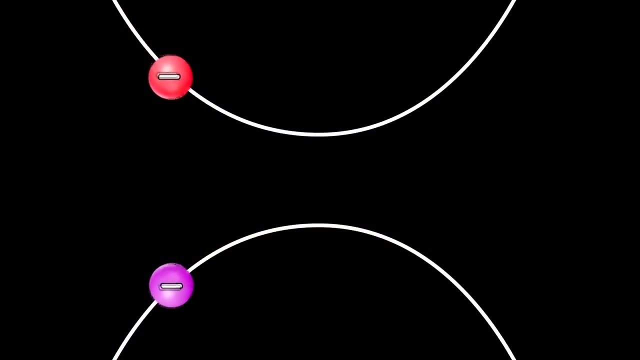 and the strong force by the gluons. In a quantum field theory, we represent each of these mediator particles with a field. For example, the photon field mediates the electromagnetic force between electrically charged particles like electrons. Other fundamental particles of the standard model are also represented by their own respective 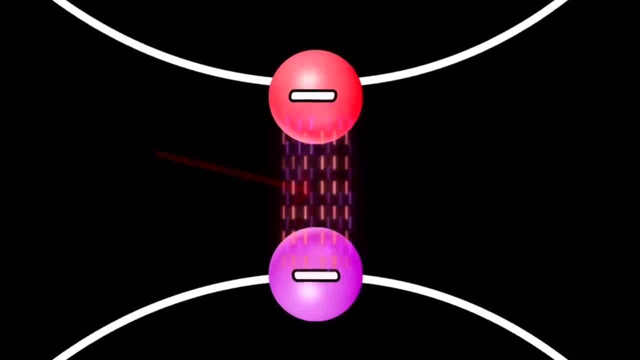 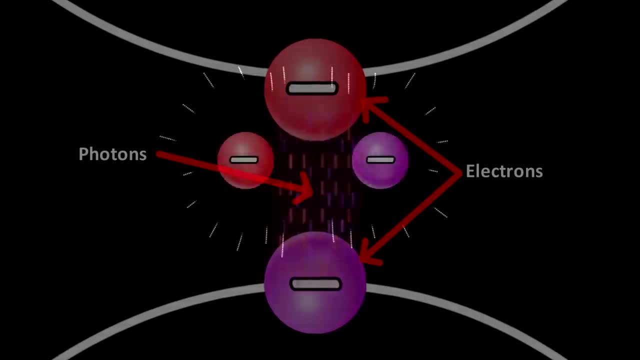 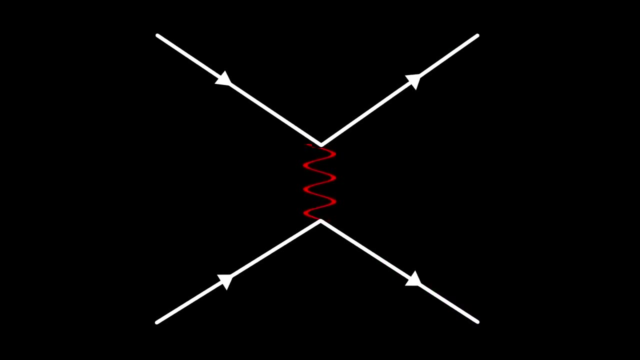 fields and these fields can interact with each other. Thus the photon field can interact with the electron field, causing a repulsion of two electrons, for example. If we generalize this concept of force-carrying particles interacting with other particles, we can get all fundamental particle physics. We can take spacetime, add a quantum field. 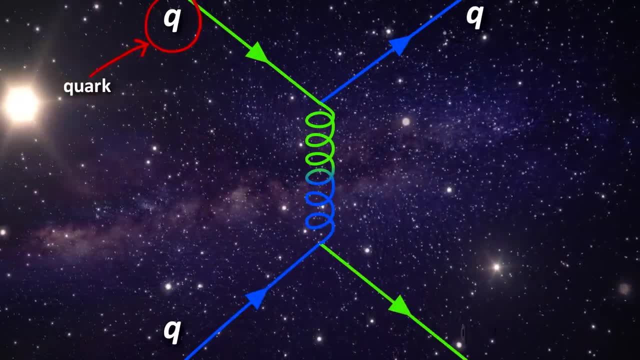 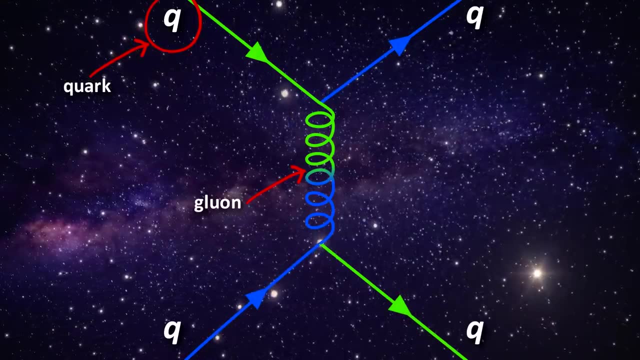 for each type of fermion like quarks. add quantum fields for appropriate bosons like gluons that mediate the force that the quark is subject to, and we can get a great representation of how it all works. These theories can be complicated, but American. 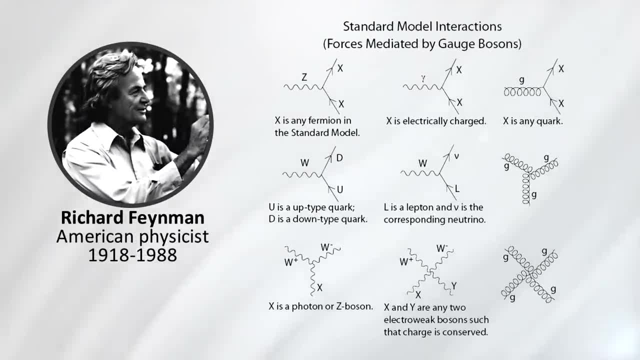 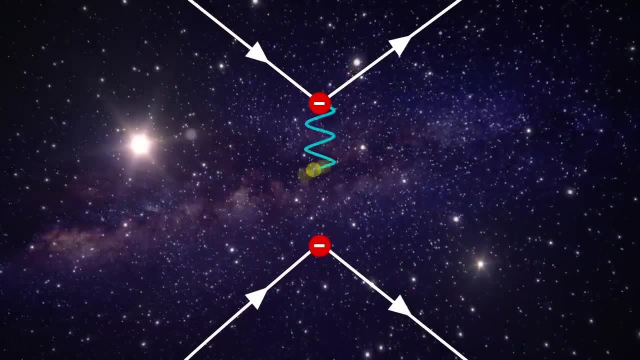 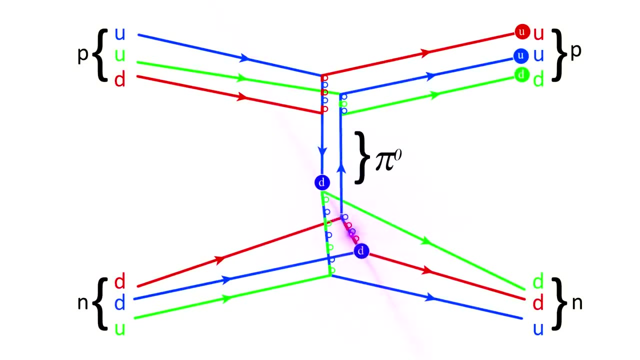 physicist Richard Feynman came up with an ingenious way to represent these interactions in what is now called Feynman diagrams. And even though these diagrams represent complicated mathematical equations, they can be visualized intuitively and drawn for any process using some simple rules If you want to understand all fundamental particle. 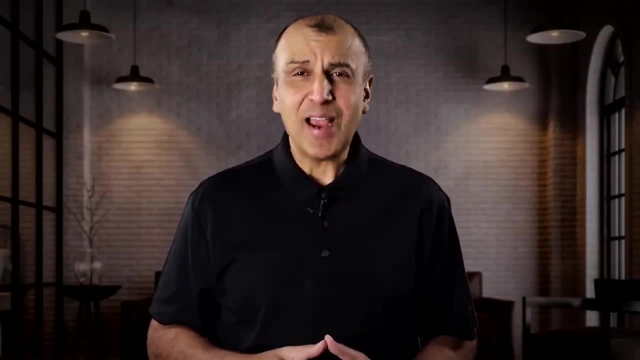 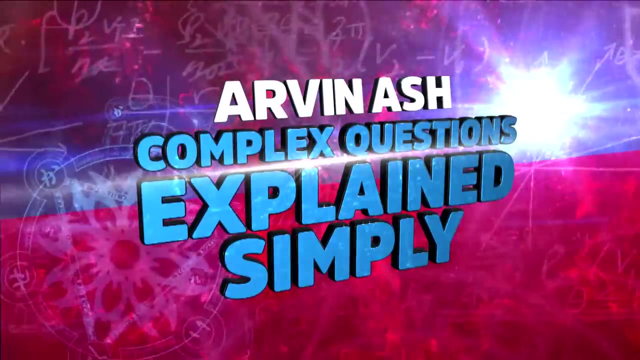 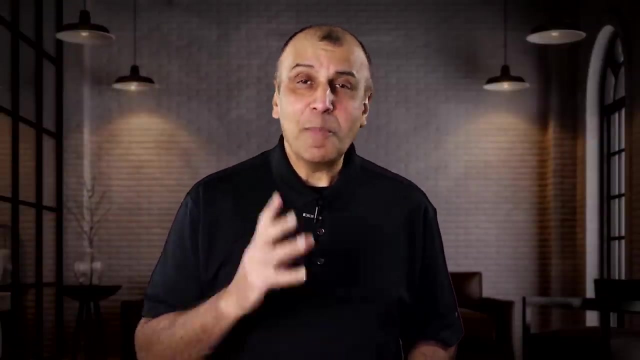 physics with the help of these simple, intuitive Feynman diagrams. then Merry Christmas, because that's coming up right now. Before we review all particle physics, I'd like to take a moment to thank MagellanTV for making this episode possible. Magellan is an ad-free documentary streaming service created. 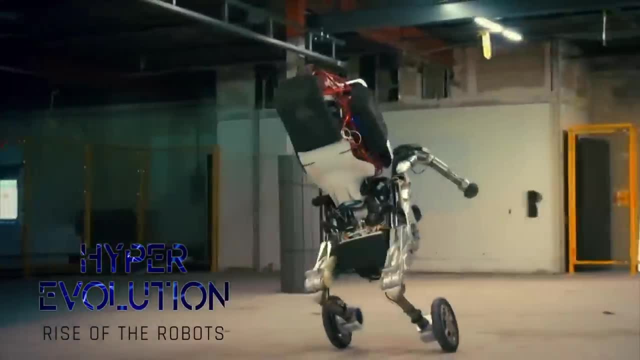 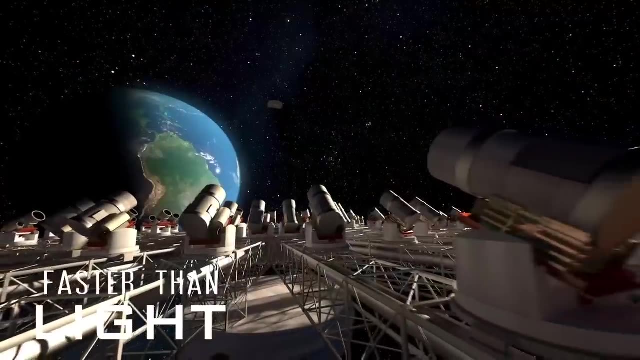 by the filmmakers themselves. Their documentary collections are richer and broader than just about any other streaming service. You can dive deep into subjects like history, culture, science and technology and see many of them in 4K. I'm excited to tell you that Magellan 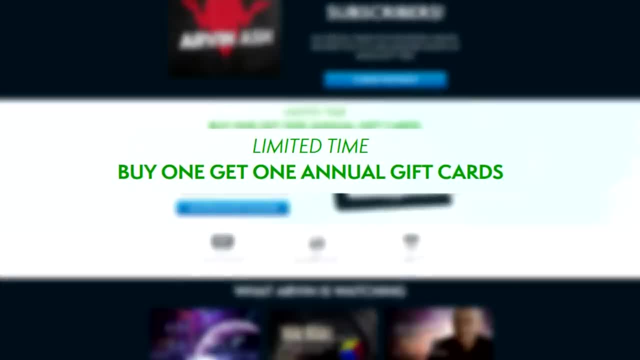 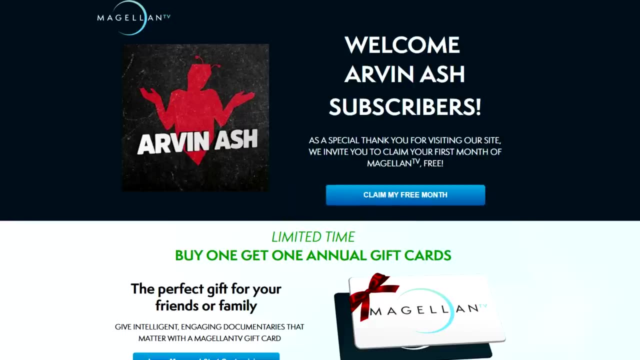 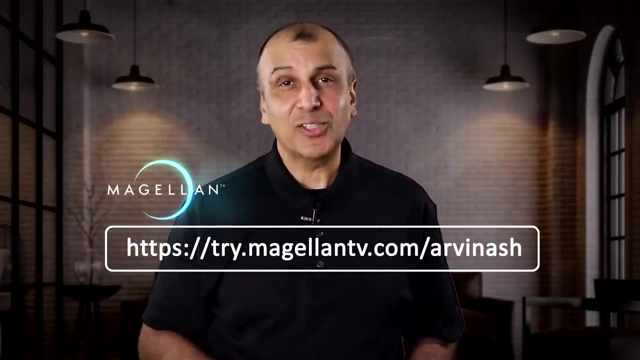 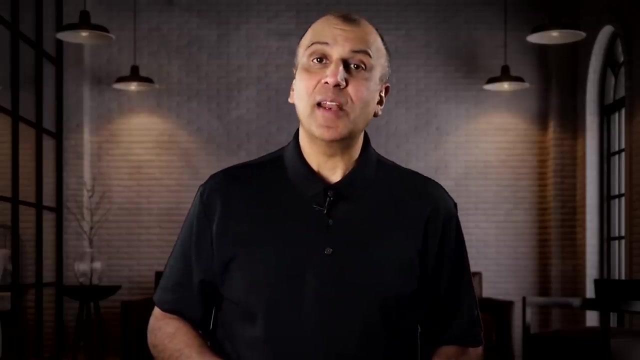 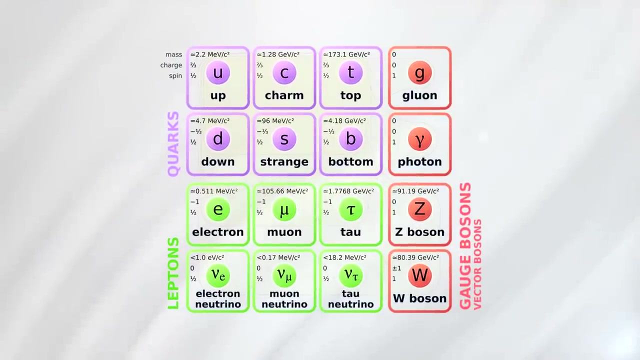 is now offering a buy one, get one free gift card for the people in your life that you want to give away. First, let's learn to make a simple Feynman diagram. To do this, we'll start with the standard model, which is like a periodic table for fundamental particles. What is important? 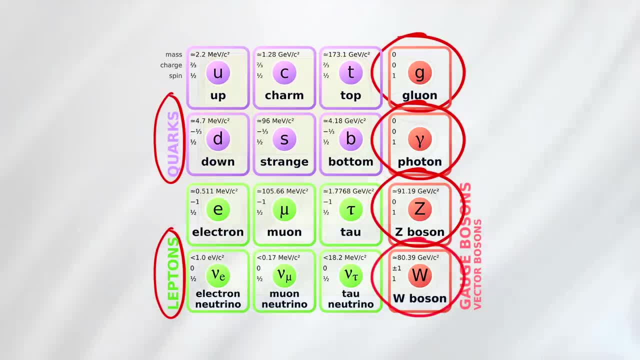 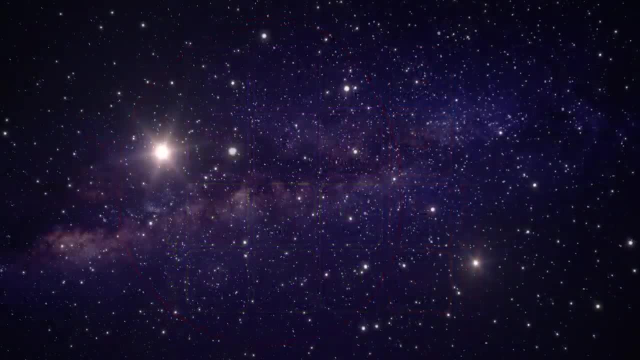 here is to understand what the different classes of particles can do. So on the left, the 12 fermions are represented with straight lines with arrows in Feynman diagrams. The arrow is important, Just like how, in an electrical circuit, the current flows. 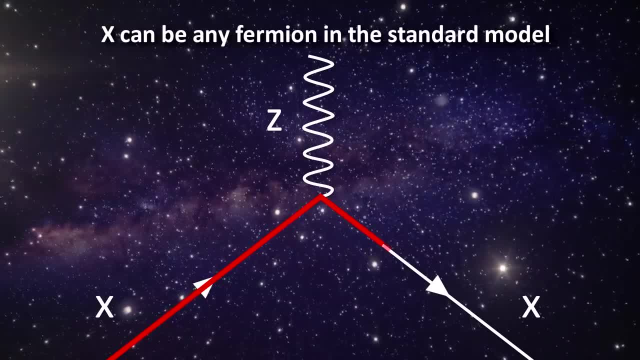 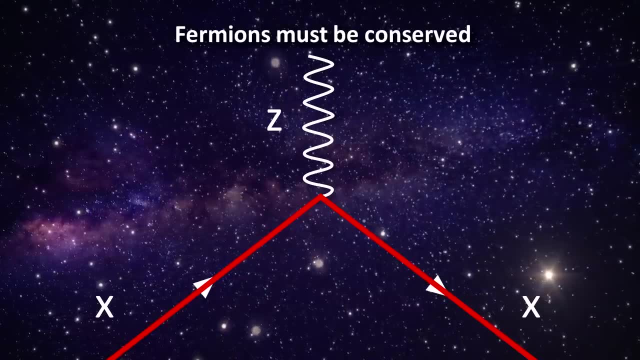 through the circuit. the arrows represent the flow of fermions. No two arrows point towards each other. This is to conserve the fermion current, or in other words, we must have the same number of fermions in the end as we started with. 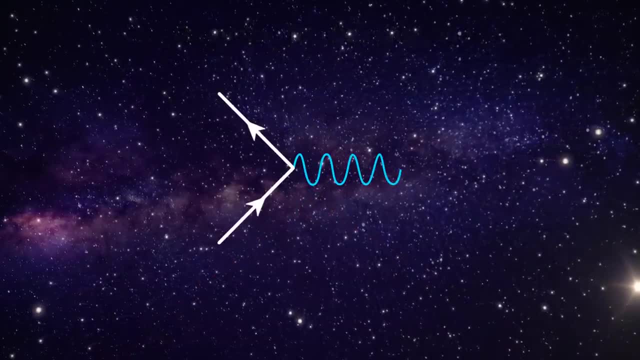 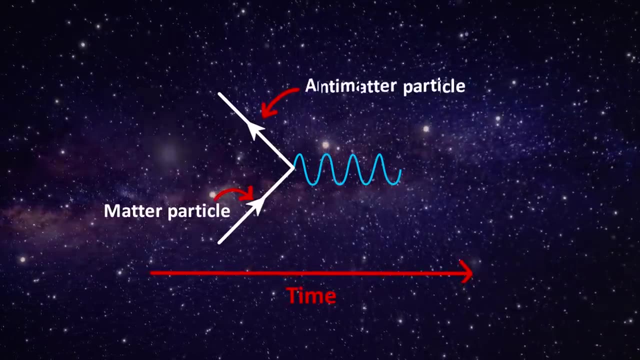 Note that there are some notations which use these arrows differently. If we consider time in the x direction, then we can interpret fermion arrows going forwards in time as matter particles and fermion arrows going backwards as antimatter particles. This is the general. 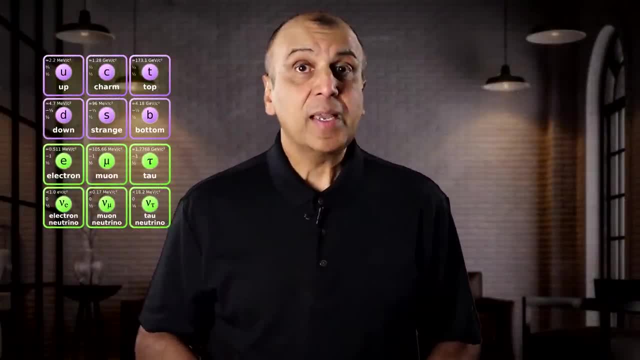 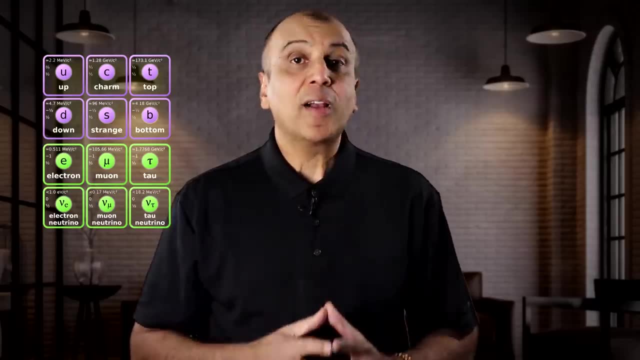 rule for all fermions. Now the fermions can be divided up further in terms of charges. When I say charges, I mean the electric and color charge. If you don't know what a color charge is, please check out my previous video on QCD. 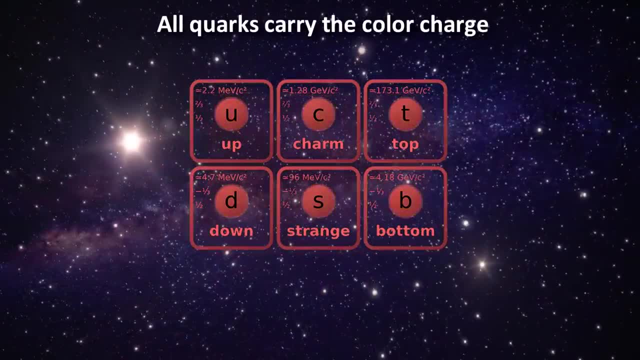 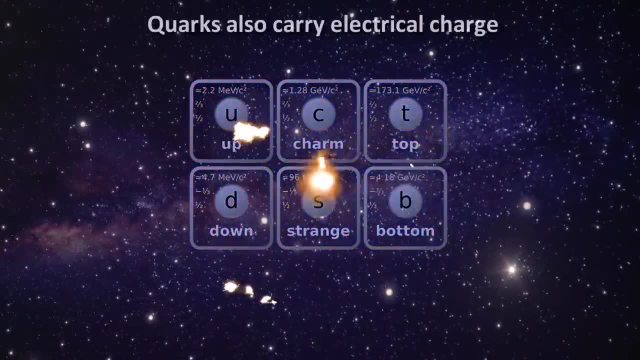 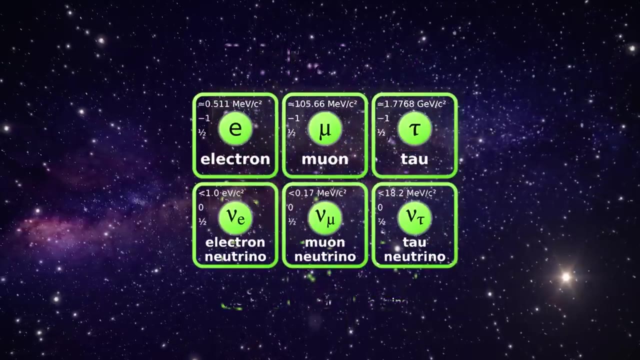 All six quarks have color charges. All particles with color charges interact with the strong nuclear force. Thus all quarks feel this force. The quarks also have an electric charge, so they also feel the electromagnetic force. The other class of fermions are the leptons. These can be divided into the electron, which 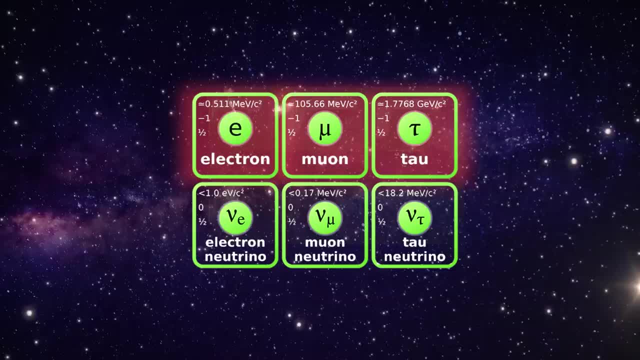 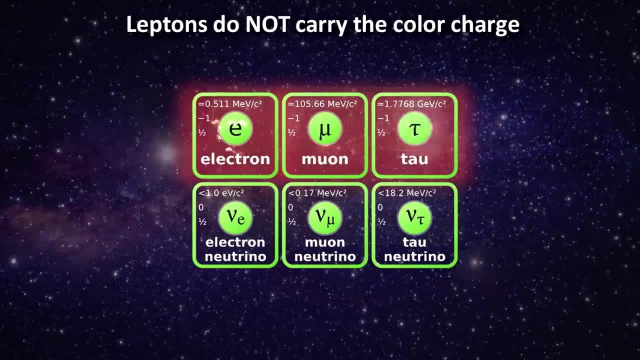 makes up an atom, and its heavier cousins, the muon and tau particles. These all have electric charges but no color charges, so they feel the electromagnetic force but not the strong force. The last three leptons are the neutrinos. These do not have a color charge. 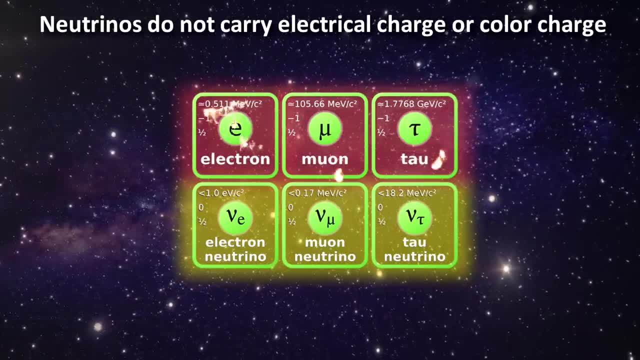 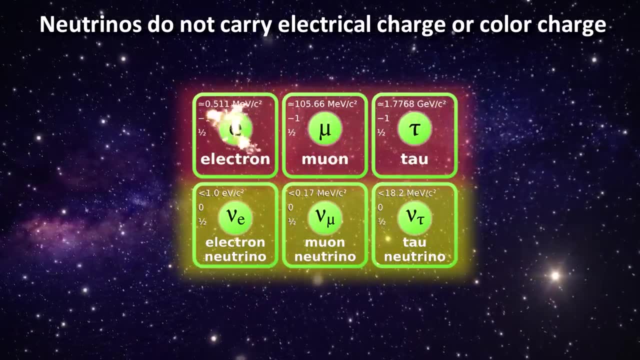 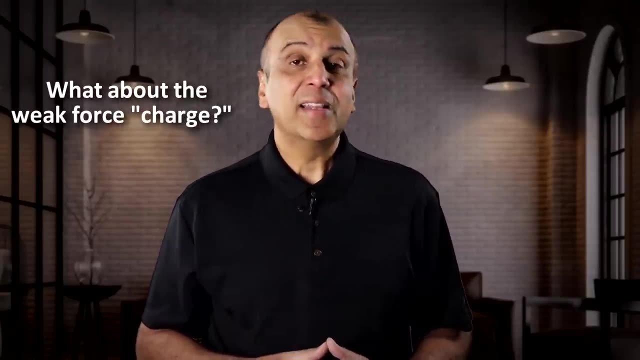 or an electric charge. Thus they are not affected by the strong or electromagnetic forces, And they have a very low mass, so they are only slightly affected by gravity. This is what makes them very difficult to detect. Now you might ask: hey, what about the weak force and its charge? The answer is that all 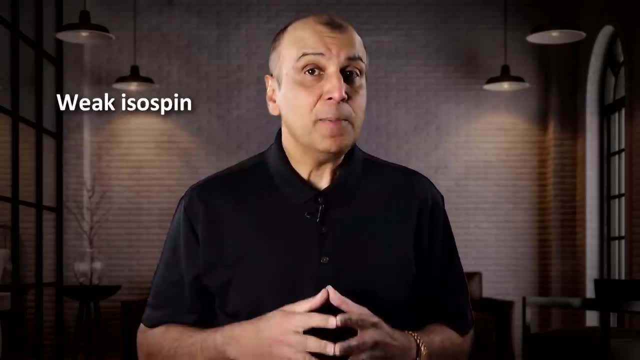 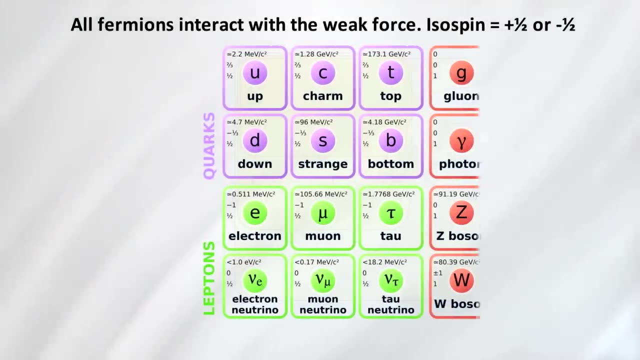 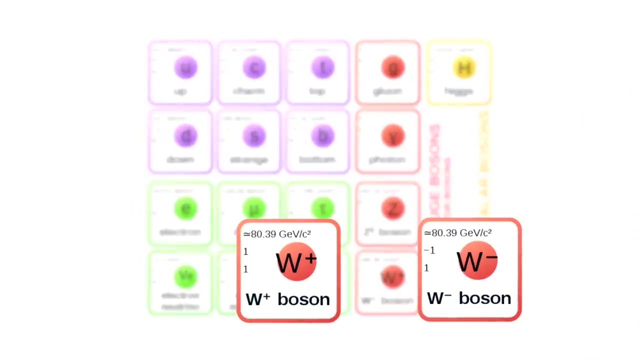 fermions carry something called weak isospen. This can be thought of as a kind of charge of the weak force For fermions. it can be plus one half or minus one half, So all fermions interact with the weak force. But weak isospen can also be negative one, zero and plus one. The W minus boson has 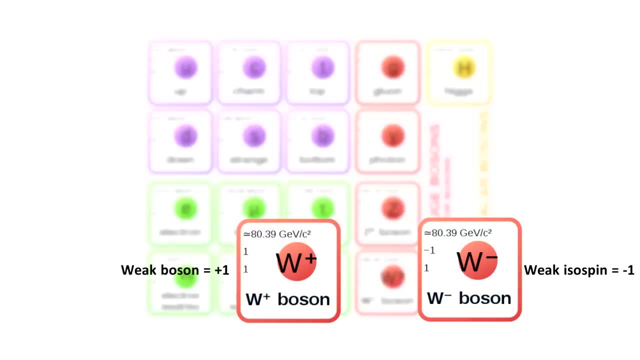 a weak isospen of negative one. W plus has plus one, Higgs has minus one half, And Z bosons and photons have a weak isospen of zero. Note that this zero is not the same as having no isospen. Both Z and photons interact with the weak force. 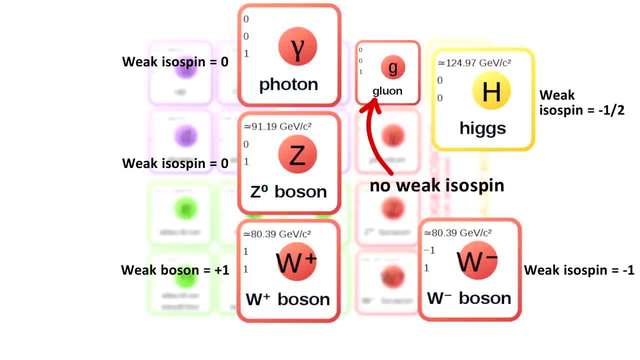 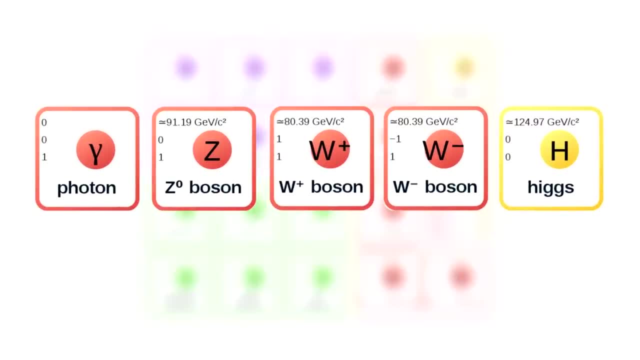 Everything in the standard model has a weak isospen except gluons. So gluons do not interact with the weak force. Weak isospen is a quantum number relating to the weak force. It's a property, just like electrical charge is a property of some particles. The number of the charge is just related to. 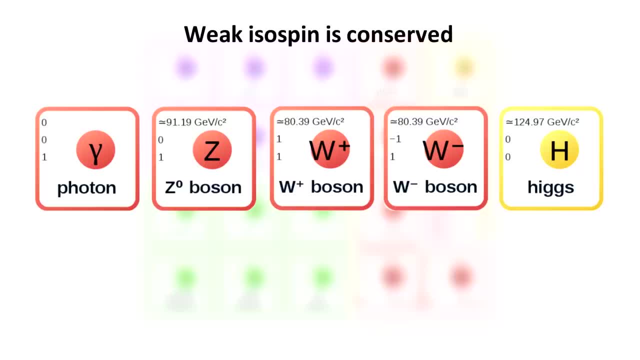 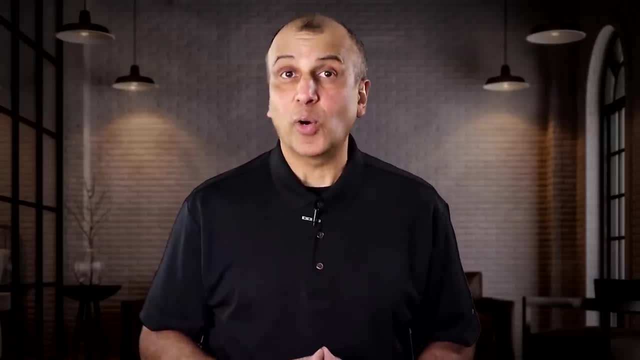 how they feel it. Weak isospen must also be conserved, Just like you must conserve electrical charge and color charge. It's a stretch to call the weak force a force. It's more like a power. The weak force has the power to turn one particle into another particle. 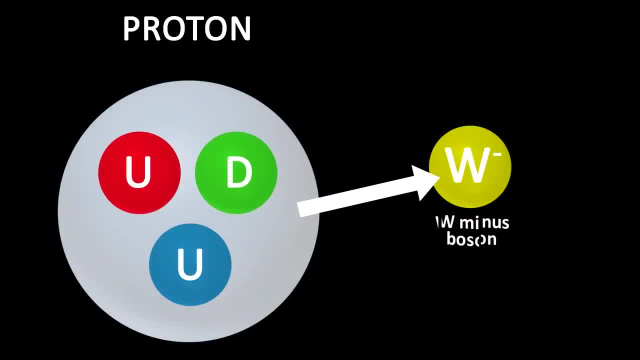 So, for example, it can turn a down quark into an up quark, turning a neutron into a proton, by emitting a W minus boson. This is the only force that can do that. Electromagnetism and the strong force can't do this. 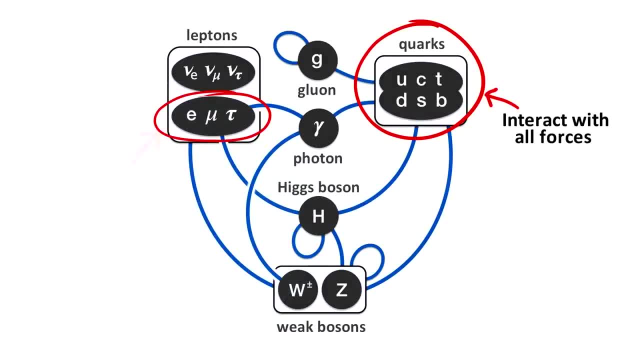 To recap, quarks interact with all forces. Electron-like particles interact with electromagnetism and the weak force, but do not interact with the strong force. Neutrinos only interact with the weak force and nothing else. Only quarks and gluons carry the strong charge. 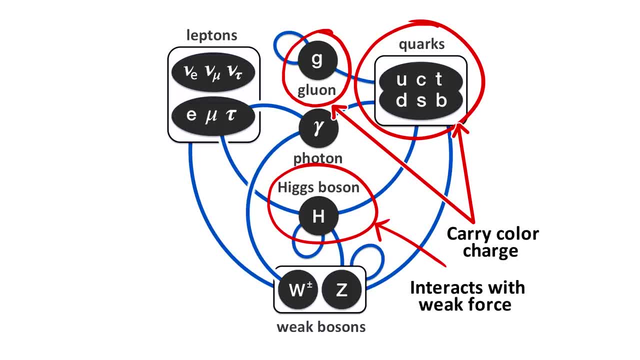 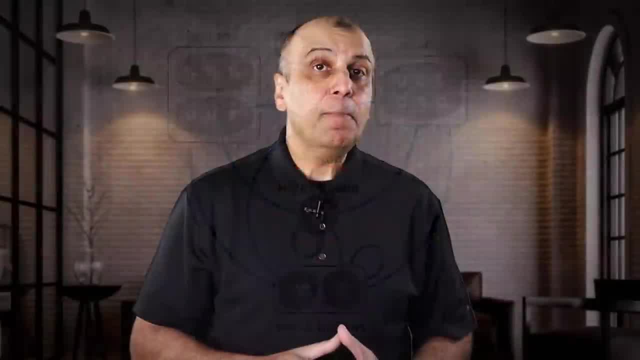 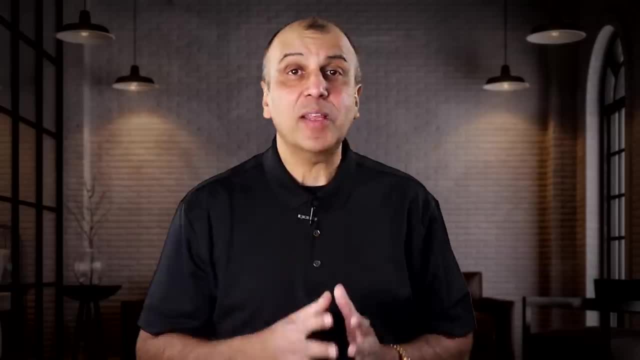 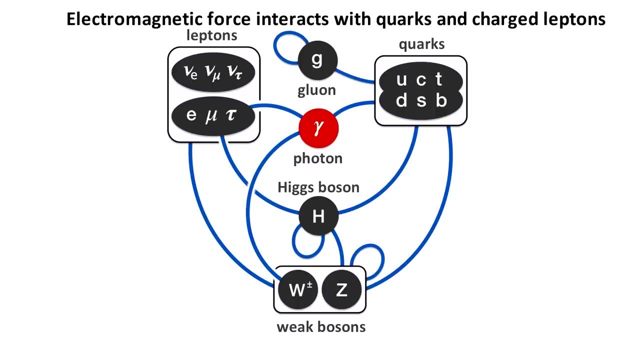 Higgs bosons do not interact with photons or gluons. They confer mass and are a very fundamental part of a residual girls classroom Manasseh's theory of environmental power around quickly generating opposite results. Higgs bosons don't interact with photons or gluons. They confer mass to fundamental particles. 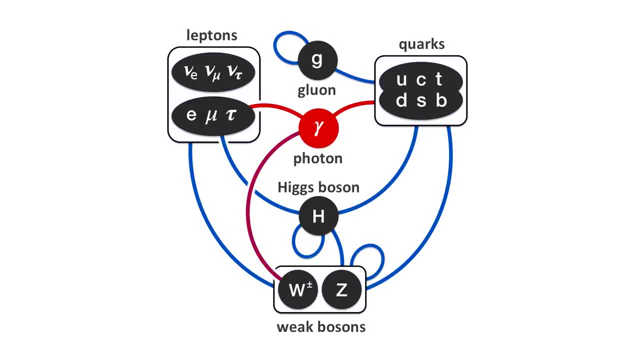 so all fundamental particles with mass interact with the Higgs. With. that have the basics needed to understand feynman diagrams. There are potentially a large number of diagrams, but we can build almost everything. Note that the W bosons, which are the mediator particles for the weak force, are charged. 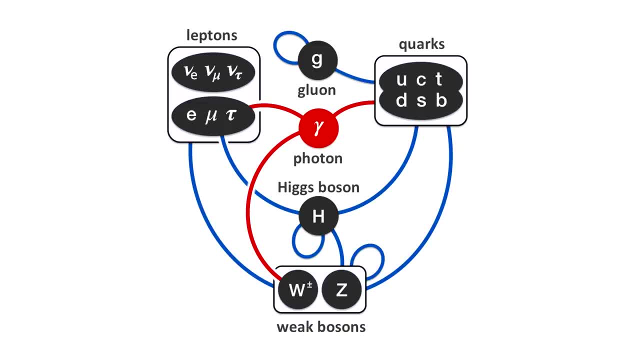 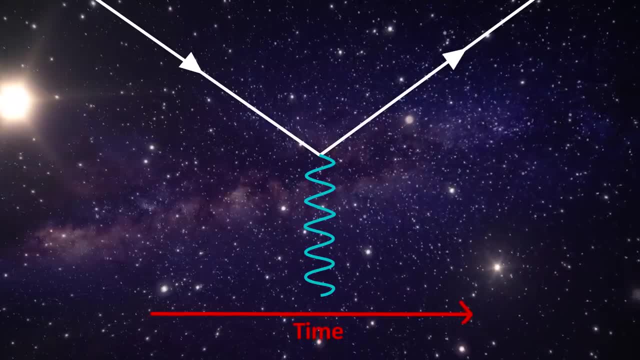 so they also feel this force, But we'll ignore them for the moment. Let's interpret one of the simplest diagrams shown here. The X axis represents time. An arrow pointing to the right represents matter- particles. There are two ways this diagram can be interpreted. 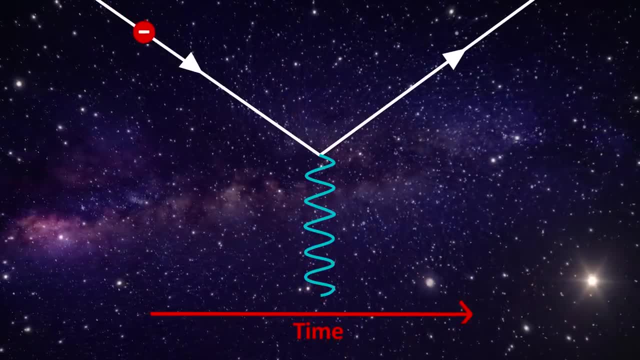 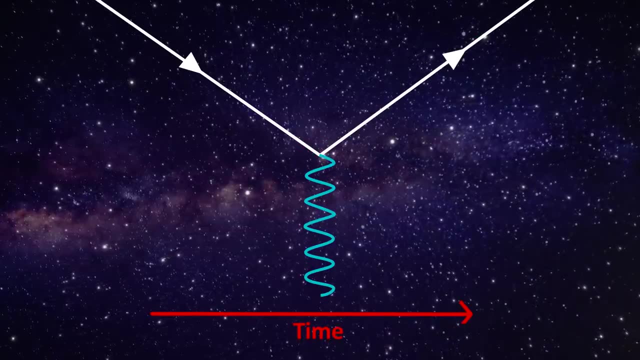 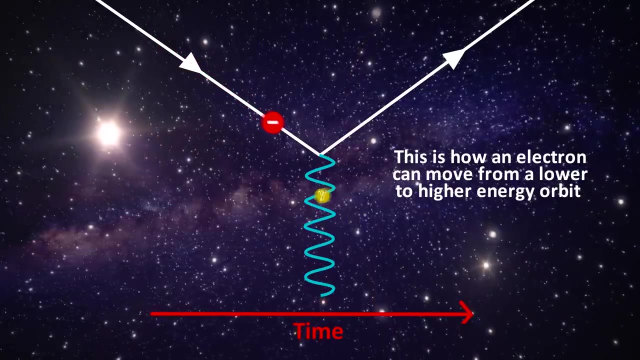 We can view it as an electron moving from left to right, while at the same time a photon moves from the bottom to top. This would depict a photon being absorbed by an electron. This is how the electron in an atom can move from a lower orbit to a higher orbit: by absorbing. 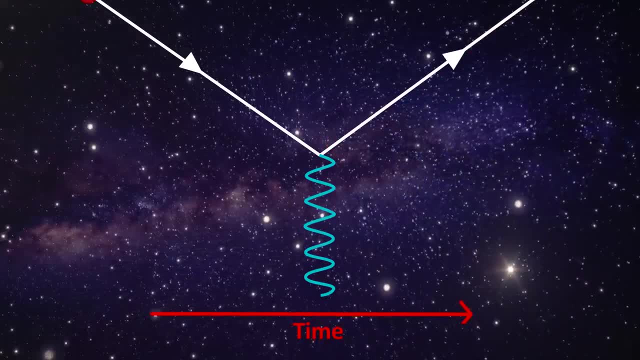 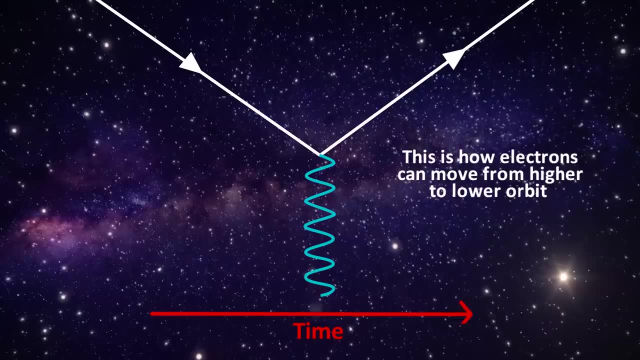 energy from the photon. We can also view this as an electron moving from left to right, emitting a photon and then continuing. In this scenario, it would represent the electron losing energy by emitting a photon. This is how an electron in an atom moves from a higher orbit to a lower orbit. 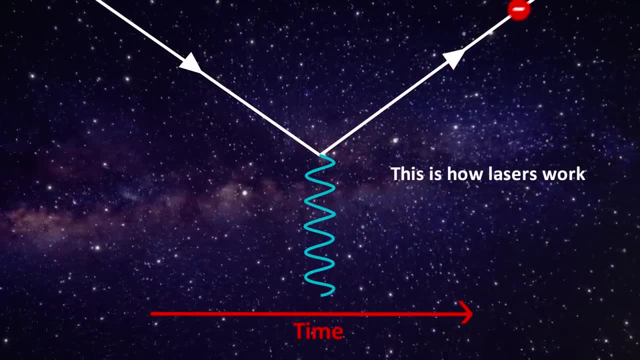 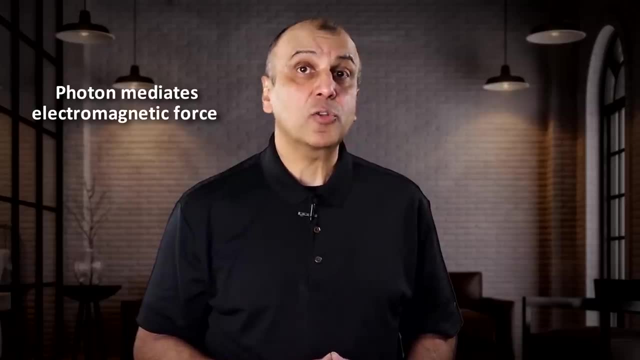 By the way, this is also how lasers work. How is electromagnetic repulsion depicted in Feynman diagrams? As we discussed, the force carrying particle for electromagnetism is the photon. This diagram, also called Muller scattering, depicts repulsion. 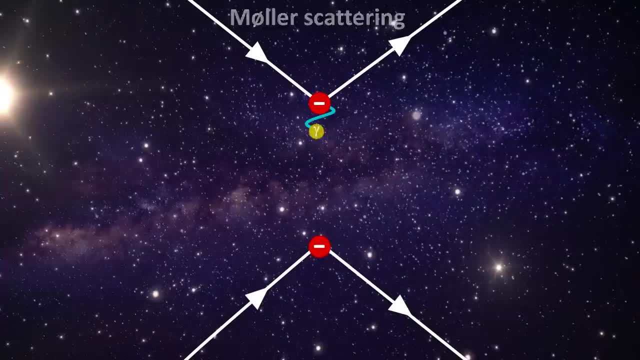 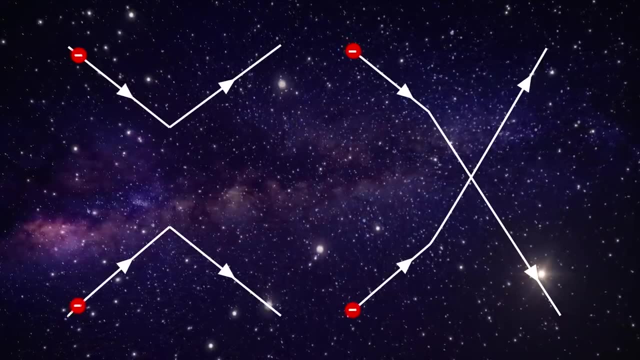 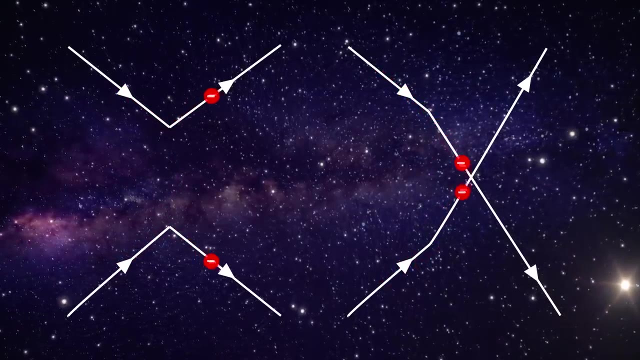 Two electrons come near each other. An exchange of virtual photons causes a transfer of momentum which pushes the two electrons apart. Note that we cannot measure the virtual photons, only the incoming and outgoing electrons. So sometimes this diagram is drawn like this: These both depict the same process. 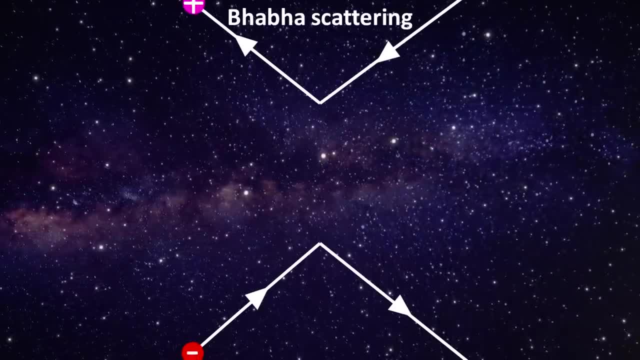 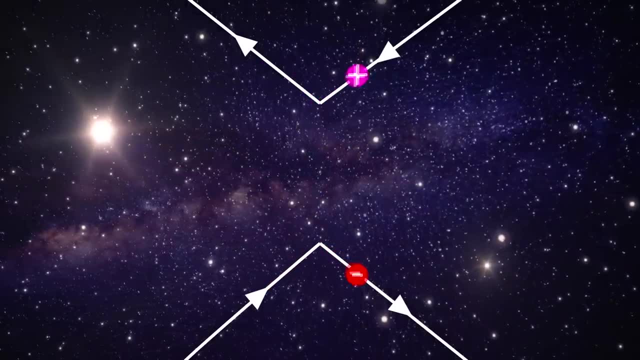 What about electromagnetic attraction? The diagram for this is called the Bhabha scattering diagram. There are two potential diagrams. The first diagram depicts an electron and positron that have opposite charges attracting each other. This also happens through the exchange of virtual photons. 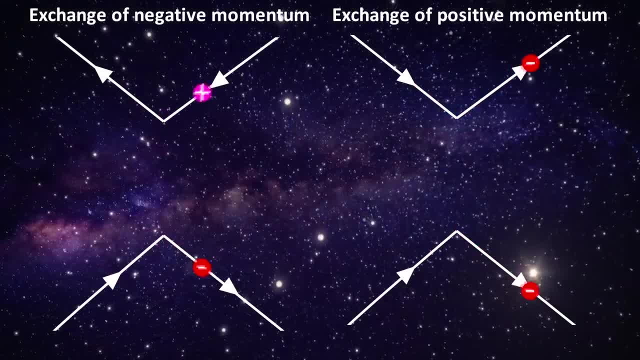 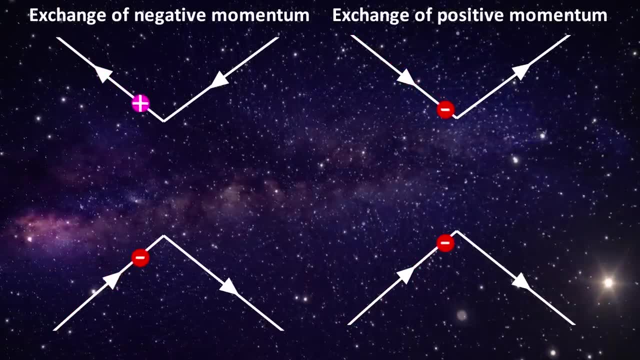 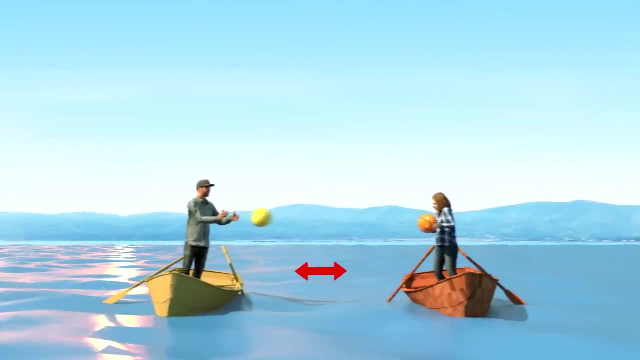 This looks very similar to the diagram for repulsion. The only difference is that the photon exchange in this case results in an exchange of negative momentum, which attracts two particles, instead of positive momentum, which repels two particles. We can see this in our boat analogy, where the boats represent electrons and the object 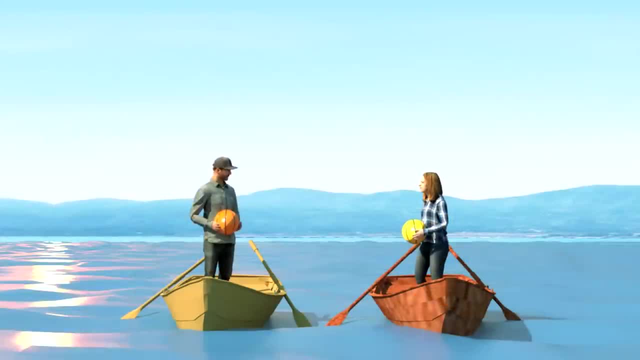 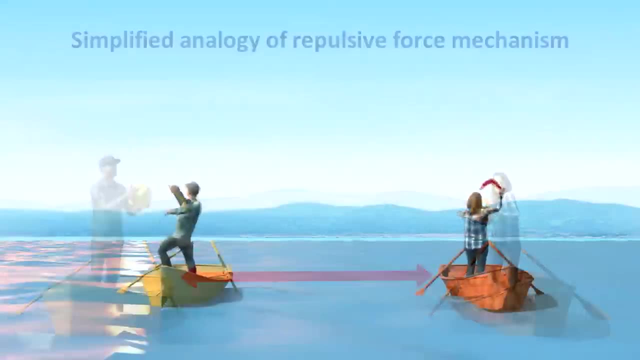 being thrown is like the virtual photon. Positive momentum exchange is like two people throwing basketballs at each other, which pushes the boats apart, But a negative momentum exchange is like two people throwing boomerangs, which results in the boats being attracted to each other. 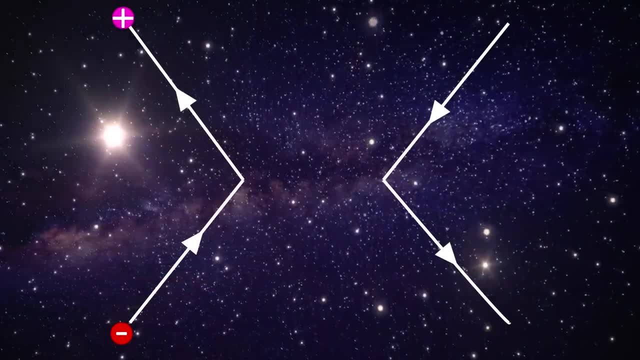 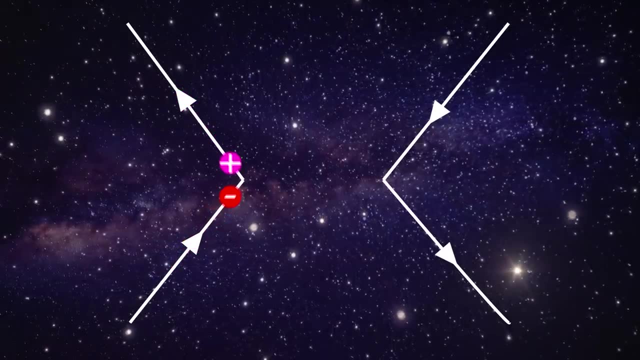 The second diagram shows a different phenomenon which can also occur when electrons and positrons are near each other. This shows that when the particle-antiparticle pair come near each other, they annihilate, resulting in energy production or photons being created. 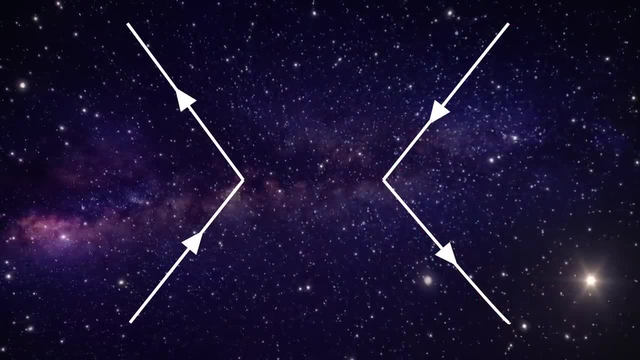 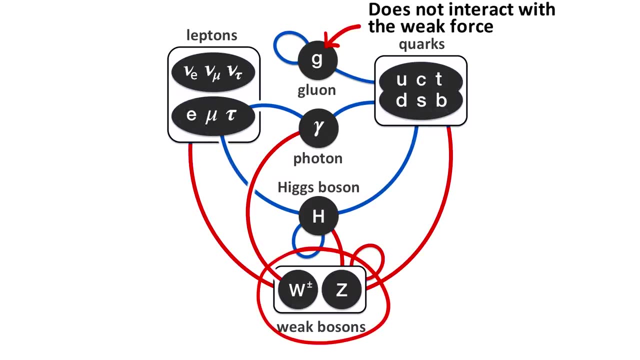 The energy of these photons in turn can create a new electron-positron pair. This leads us to the slightly more complicated weak force. This force is felt by all the standard model particles except gluons. The most interesting weak force diagrams involve…. 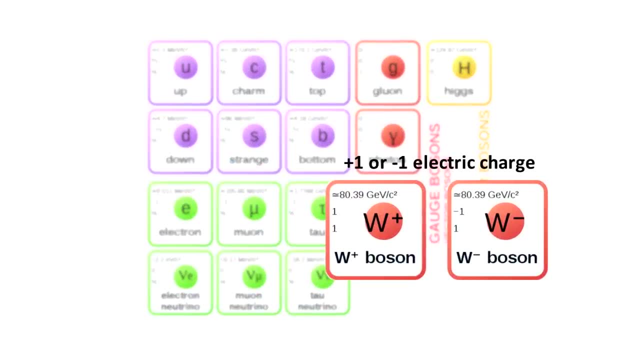 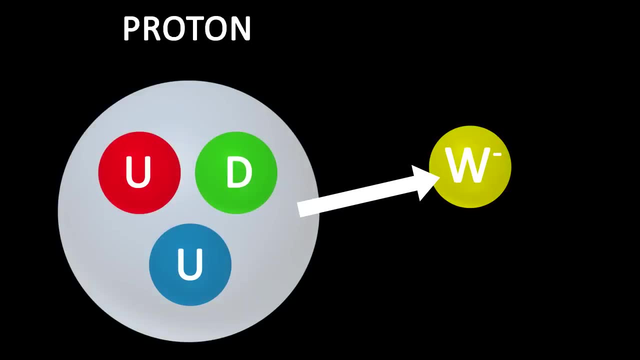 W bosons which can have a plus one or minus one charge. These particles can do something very special. They can change the identity or flavor of a particle. For example, they can change an up quark into a down quark. This is so important that we probably would not exist without it. 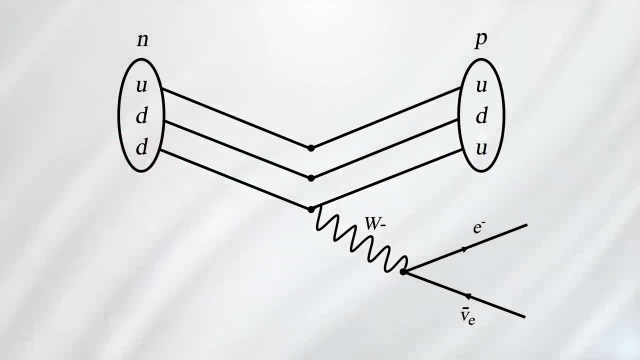 So, for example, here is one of the most important weak force interactions relevant to life. This involves a neutron decaying into a combination of a proton, electron and antineutrino. On the left side we have a neutron which is composed of one up quark and two down quarks. One of the down quarks can change flavor and become an up quark. This happens due to the W- weak force mediator particle. When the W boson is emitted, the down quark changes its flavor to an up quark. This W- boson then almost immediately decays into an electron and an antineutrino. 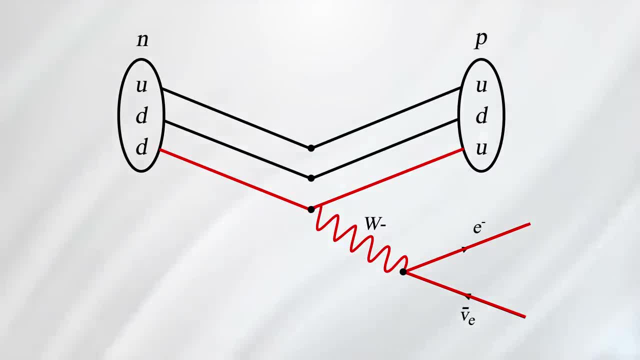 Because the new particle now has an up quark and a down quark. the down quark can change its flavor and become an up quark. When the W boson has two up quarks and one down quark, our original neutron has turned. 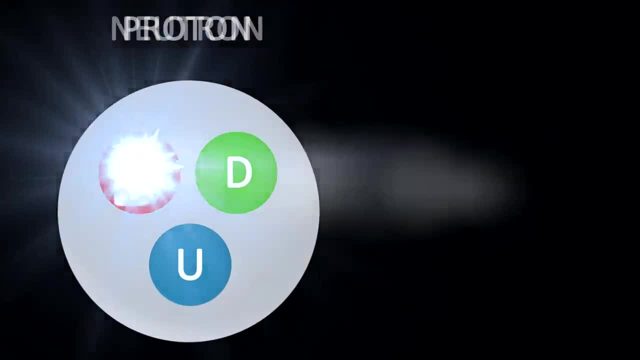 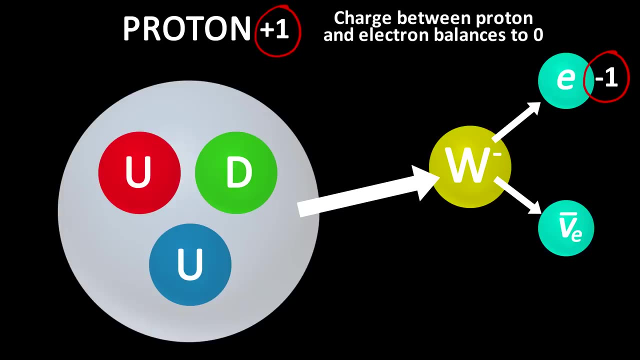 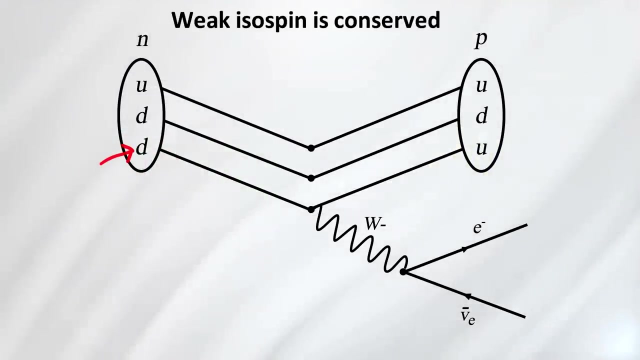 into a proton. Note that charge is still conserved because the emitted negative charge of the electron is balanced by the positive charge of the proton. And weak isospin is also conserved because the isospin change of plus one created when a down quark changed to an up quark, is balanced by the combined minus one spin of the electron. 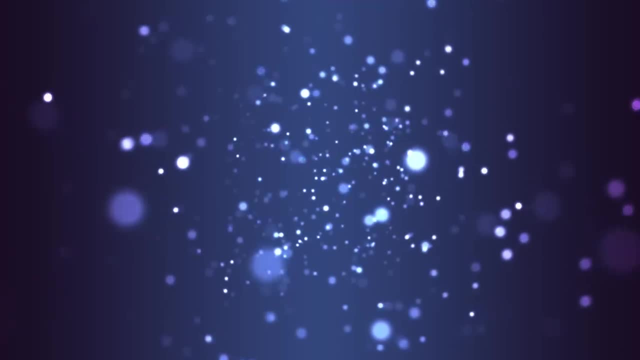 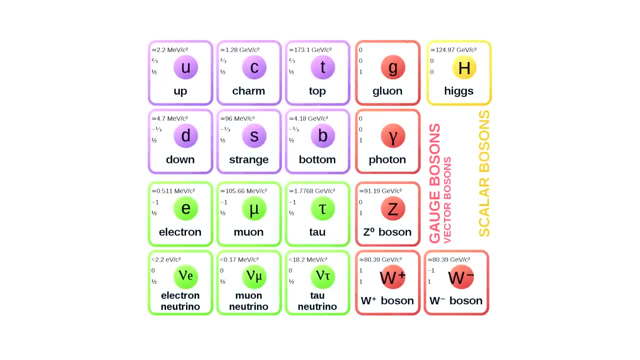 If this decay did not occur, the early universe may have been awash in neutrons and atoms may never have formed. Another interesting weak force interaction involves a Z boson. It has no electric charge, just like the photon, but unlike the photon it can mediate interactions. 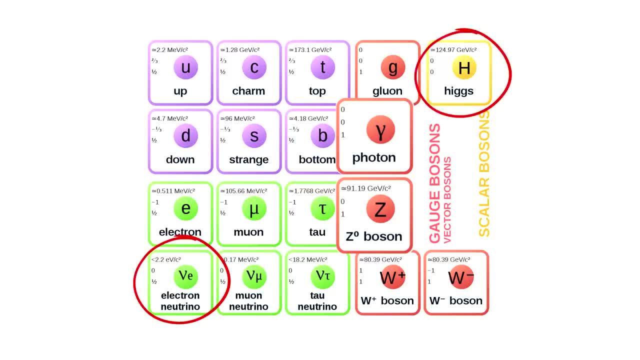 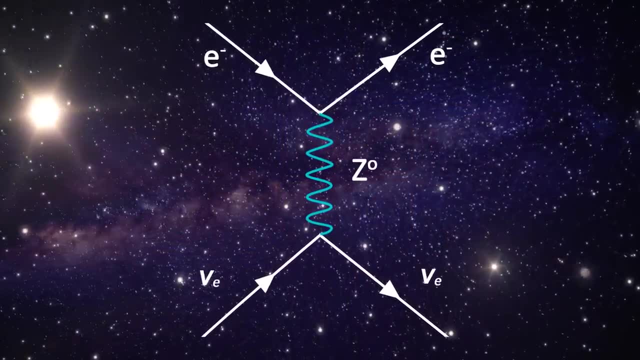 with electrically neutral particles like the neutrino and Higgs. So for example, as the Feynman diagram below shows, a Z boson can transfer spin and momentum between an electron and a neutron, But in the process of doing so it does not transfer any charge and leaves the particles. 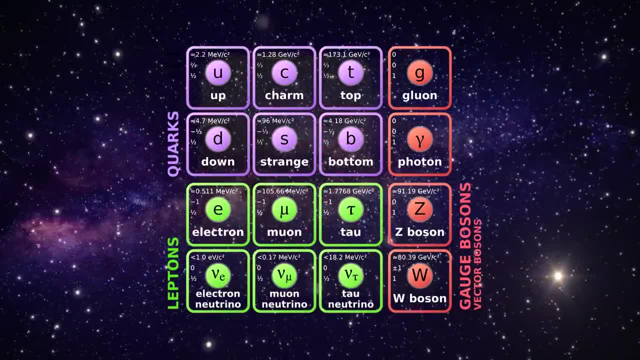 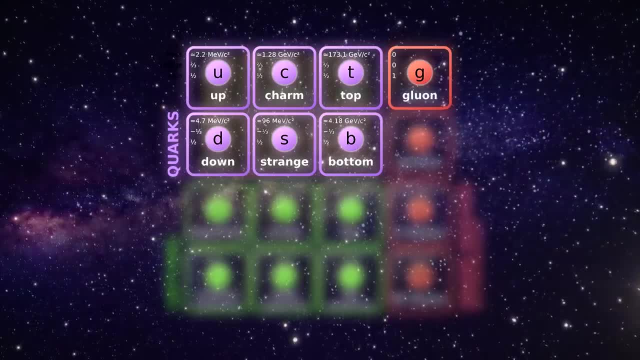 otherwise unaffected. This brings us to the strong force, which is the most complicated mathematically, but since it only relates to quarks and gluons, there are fewer interactions to understand. One of the simplest diagrams is the quark interaction diagram. 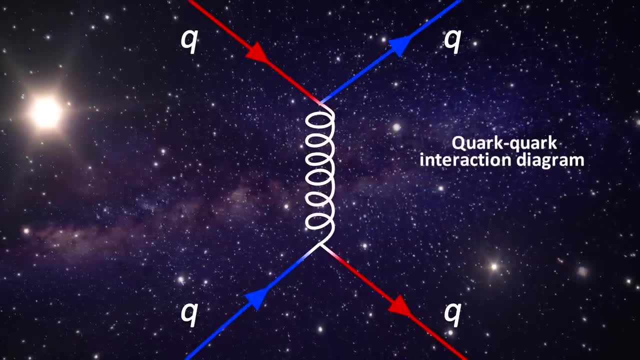 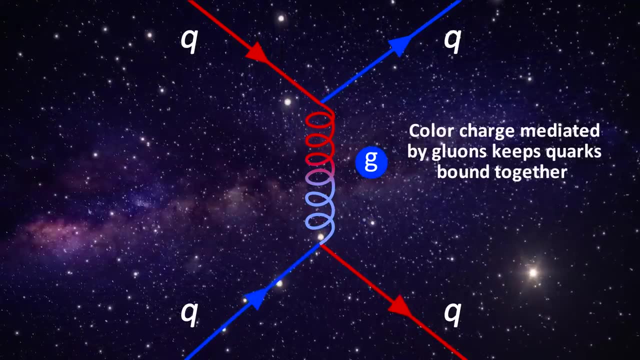 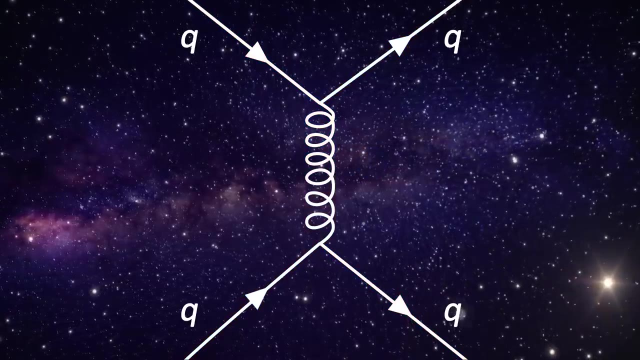 Here, a pair of quarks simply change color. This process happens all the time inside protons and neutrons, And this color charge exchange is the glue that binds the quarks together and keeps them confined to the inside of nucleons. A blue and red quark, for example, can change colors via the exchange of a gluon. 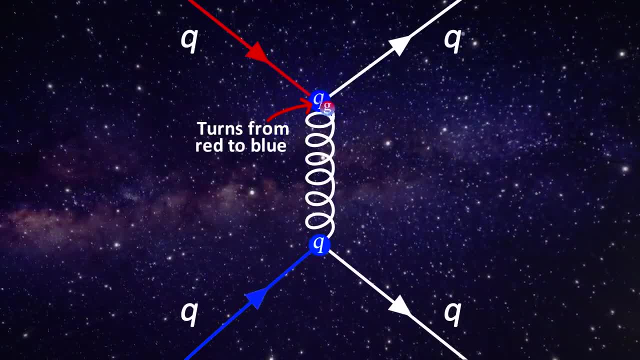 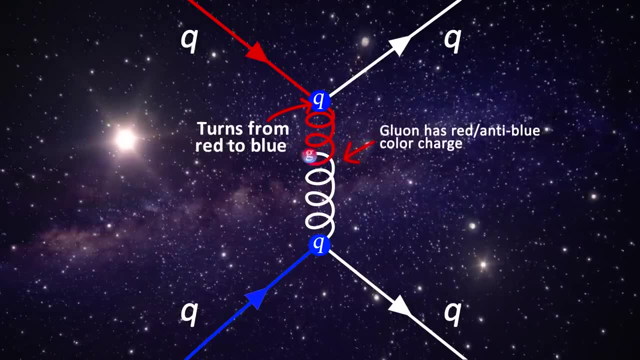 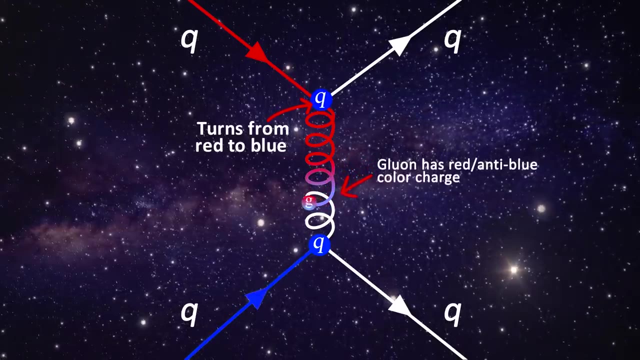 So on this diagram we have a red quark. coming from the top left. It emits a gluon with a combination of red and anti-blue color charge Gluons always have a combination of color anti-color charges. The outgoing anti-blue of the gluon immediately turns the quark into a blue quark. 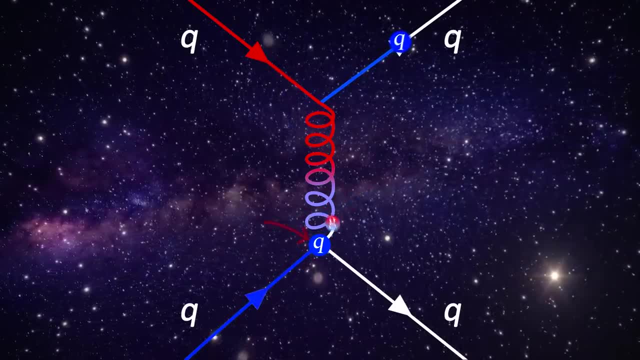 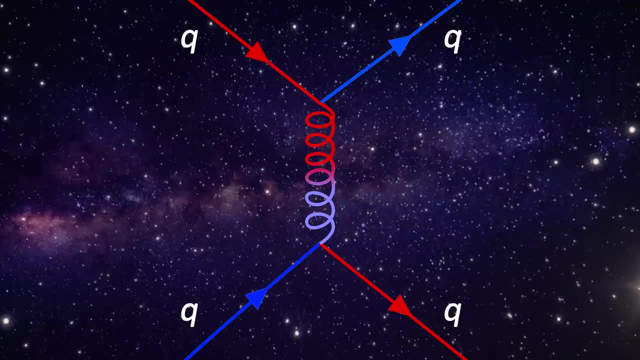 The blue quark at the bottom absorbs this gluon. This blue color gets neutralized by the anti-blue contained in the gluon And this quark turns red by absorbing the red that was also part of the gluon. Note that color is conserved in this interaction. 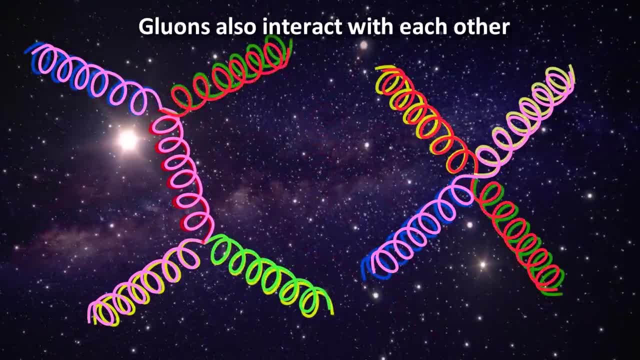 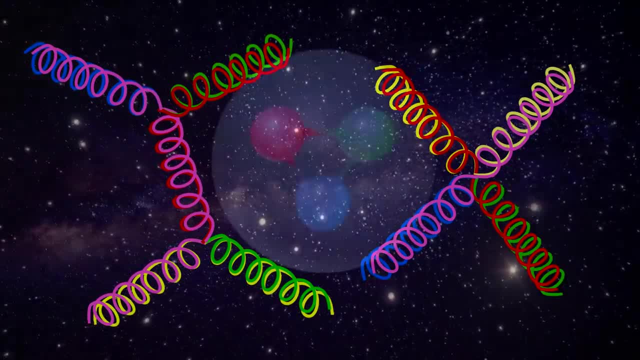 Because gluons themselves contain color charges. they also interact with each other via complicated diagrams. These gluon-gluon interactions is what the flux tubes inside nucleons are made of. These tubes are formed when you try to pull quarks together. The flux tubes are formed when you try to pull quarks together. 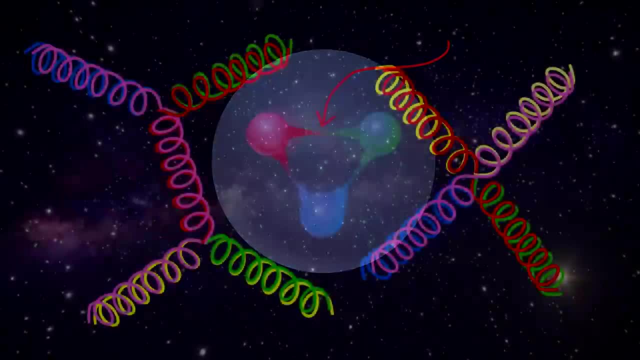 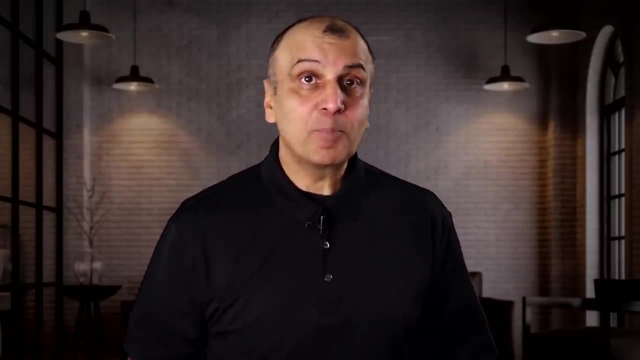 This process is calledomenant For every single skull. justement, the glucose in the glucose takes a very new form, the mercury, and can break quarks apart, as discussed in a video about QCD. Now lets look at what is the most complicated Feynman diagram in this video, but may very 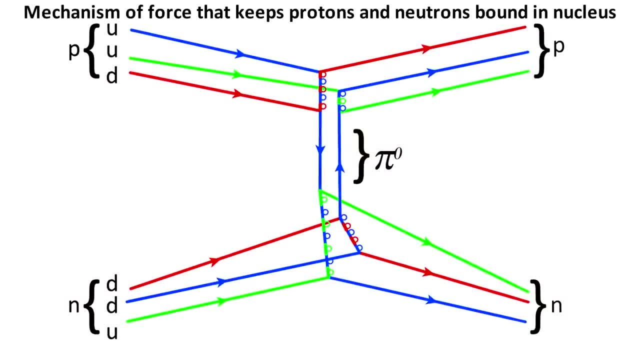 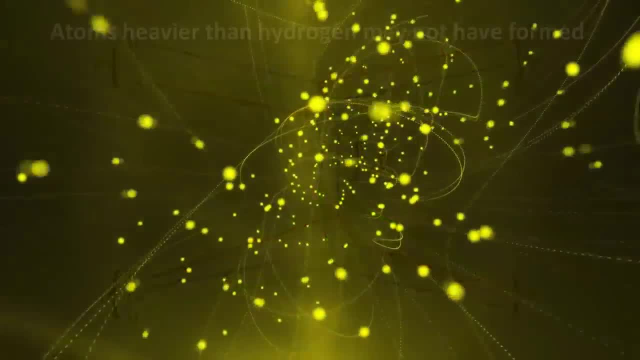 well also be the most important. This diagram represents the strong force interaction that binds protons and neutrons together in the nucleus. Without this interaction, there would be no atoms heavier than hydrogen, and life as we know it would not exist. What happens now without this interaction, is that changedyluxon is bound together with 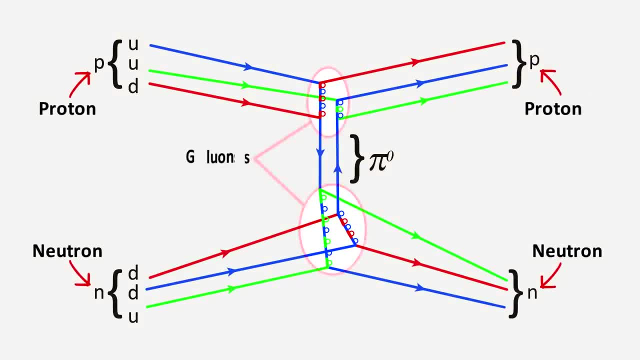 a particle in the nucleus called, in which an atomic atom would work continuously and proton and neutron interact with each other via gluons, yielding some residual energy, which becomes mesons. These mesons are a combination of quark-antiquark pairs. These in turn mediate. 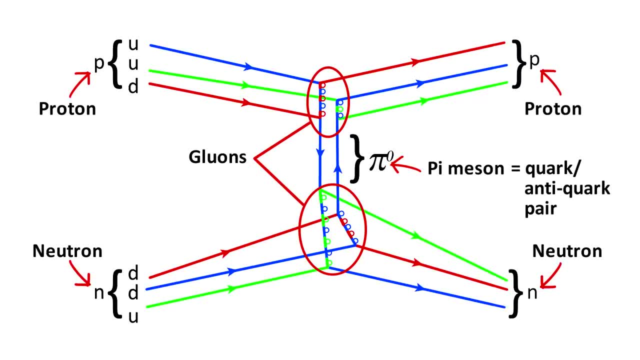 the strong force between the proton and neutron. Let's take a close look at exactly how this attractive force works. We have a proton up top and a neutron at the bottom. Keep in mind that color must always be conserved. That is, the three quarks inside. a proton or neutron must be a combination. 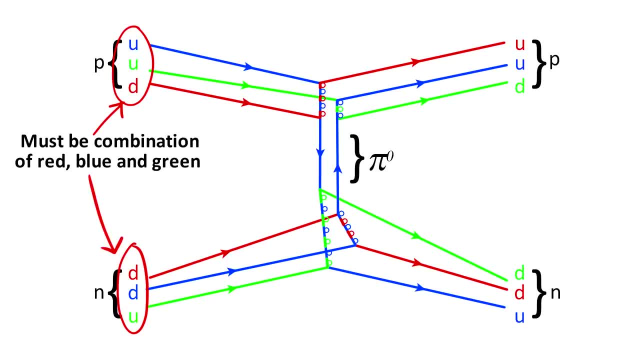 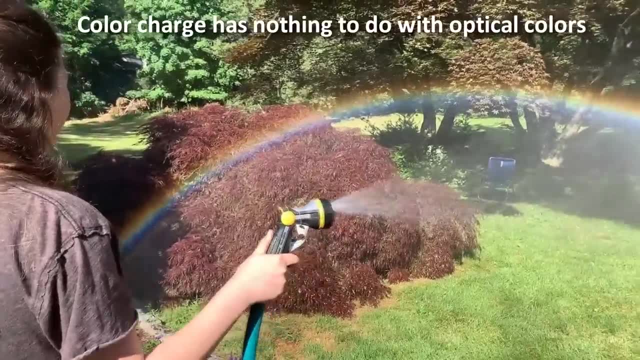 of red, blue and green, which combine to make a neutral white color. Let me clarify that this is the same way that optical colors combine, but color charge is a metaphor and has nothing to do with colors that you can see with your eyes. 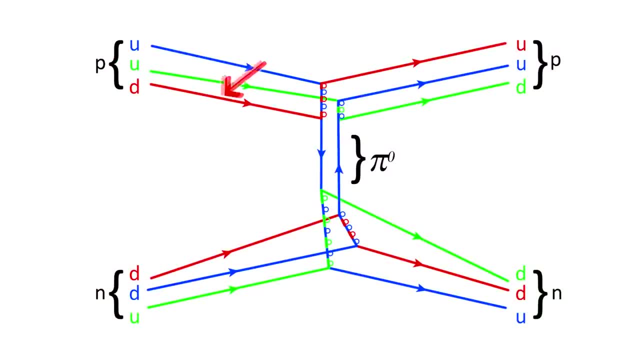 Inside the proton, the blue up quark interacts with the red down quark via a gluon. This turns the up quark red and the down quark blue. As this down quark leaves the proton, an anti-blue, anti-quark is created. 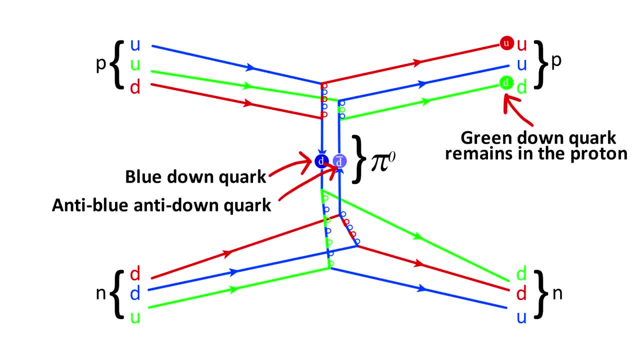 together with a green down quark via a gluon interaction between the green up quark, which was initially green but now turns blue, The blue down quark and the anti-blue. anti-down quark leaves the proton forming a charge and charge neutral, pi-meson. Meanwhile, the newly created green down quark in the proton 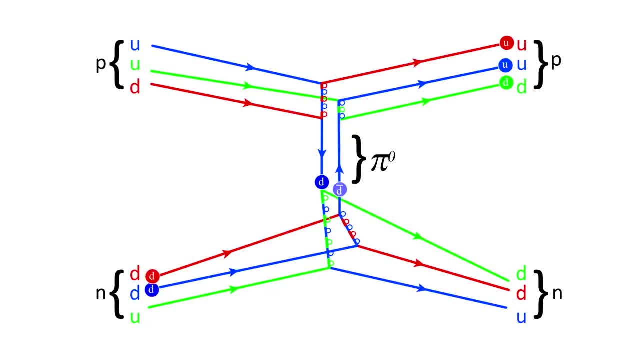 remains in the proton. The pi-meson now interacts with the neutron. The anti-down quark of the meson annihilates the down quark of the neutron. At the same time, there is a color exchange between the red down, blue down and anti-blue, anti-quark, such that the quark which is not 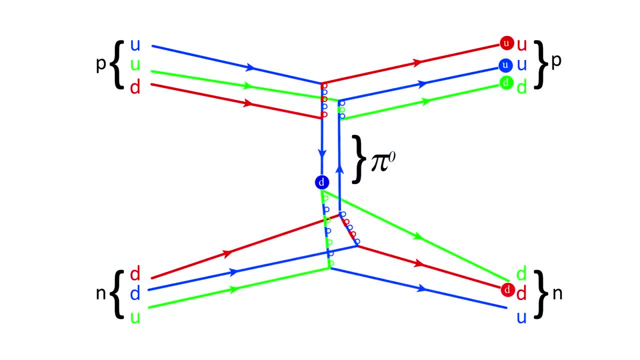 annihilated becomes red. The down quark of the meson joins the neutron by taking the place of the annihilated down quark. At the same time, an exchange of colors occurs with the green up quark of the neutron, such that the up quark turns blue and the blue down quark changes to blue. 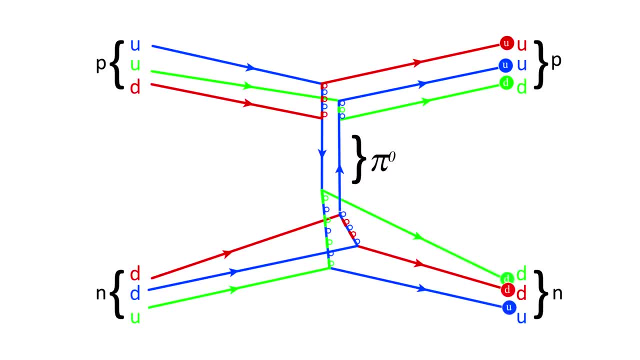 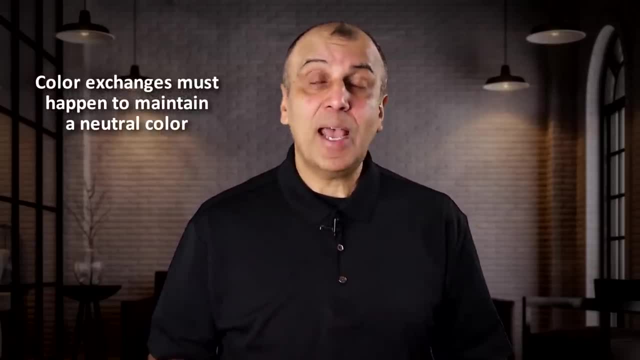 and the new dawn quark from the pie meson turns green. You might ask: why are there so many color changes happening in this interaction? The color exchanges have to happen in order to maintain a neutral color charge in both the proton and neutron. That's the way quantum chromodynamics works. It can't work without. 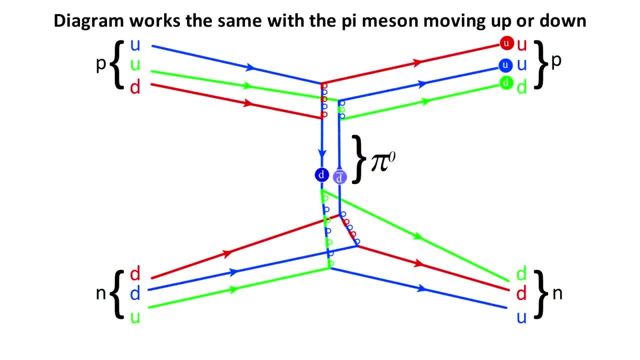 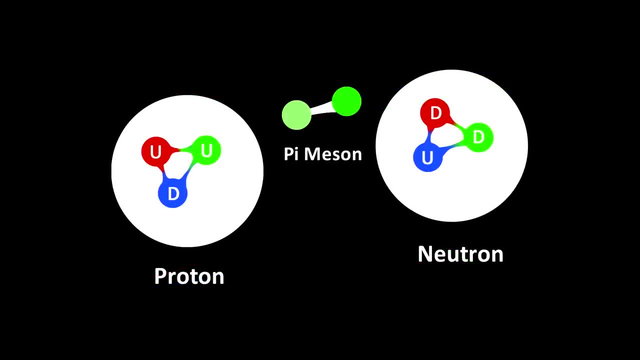 it. Note that this interaction works equally well both ways, whether you go up or down. Also note that these virtual meson interactions are what keep protons and neutrons bound together in atoms, But the attraction is much weaker than the gluon interactions that keep the 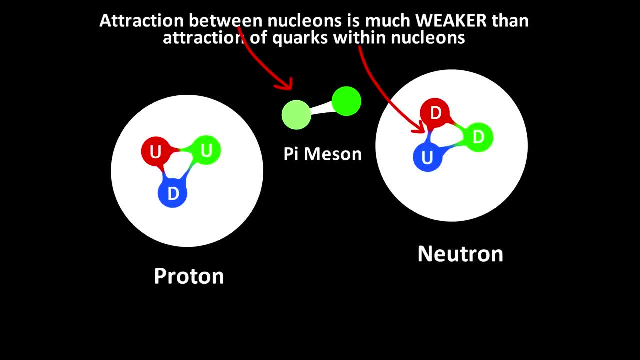 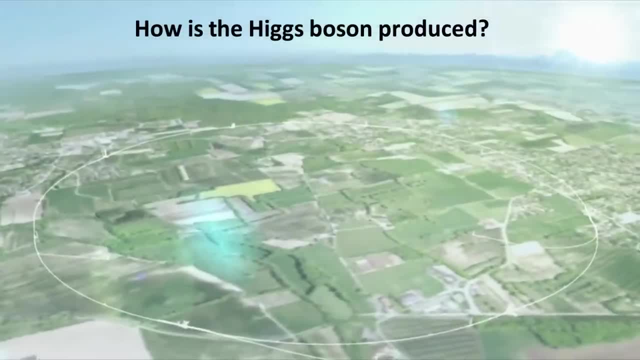 quarks within the nucleons and they work only at short distances much smaller than the width of a proton. The last thing I want to show you is how physicists produced the long sought after Higgs boson. While there are several ways it can be made, the most prominent process used at the Large 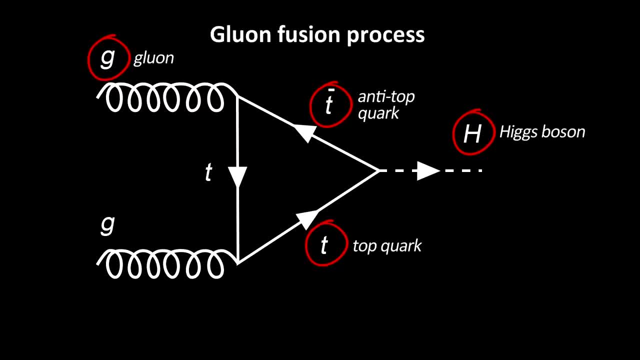 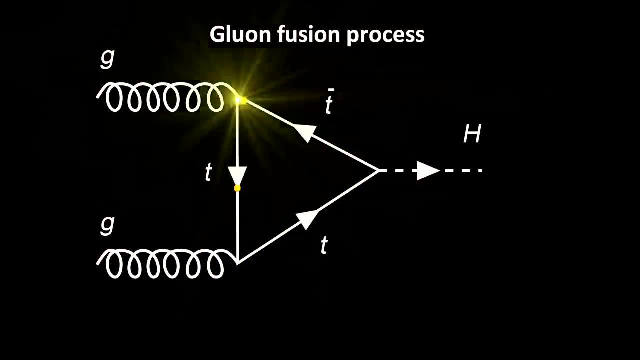 Hadron Collider is the so-called gluon fusion process. What happens is that in some high energy proton-proton collisions at the LHC, two high energy gluons can be produced. These can, in some cases, due to strong force interactions, turn into top quarks and fuse together via a triangle loop. The 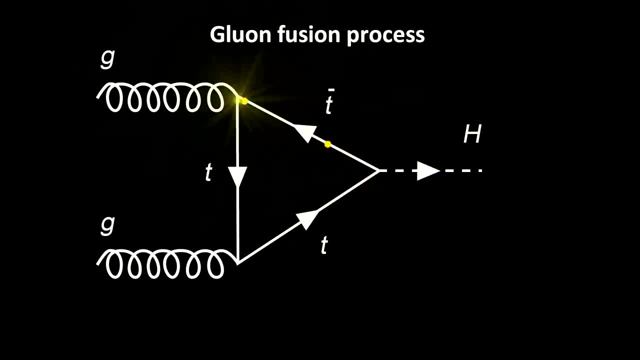 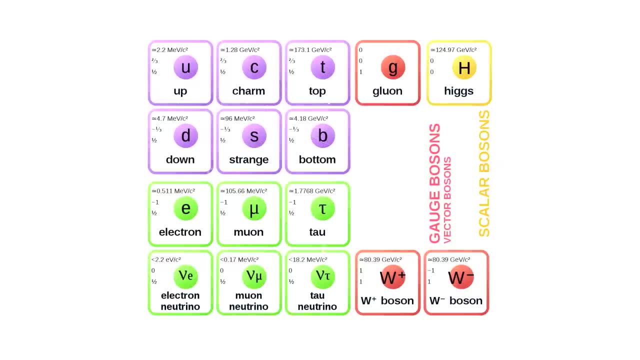 loop represents top quark-anti-top quark creation and annihilation. The energy of this annihilation can create a Higgs boson. Because the top quark has the highest mass of all elementary particles, it has the best chance to decay into a Higgs boson. 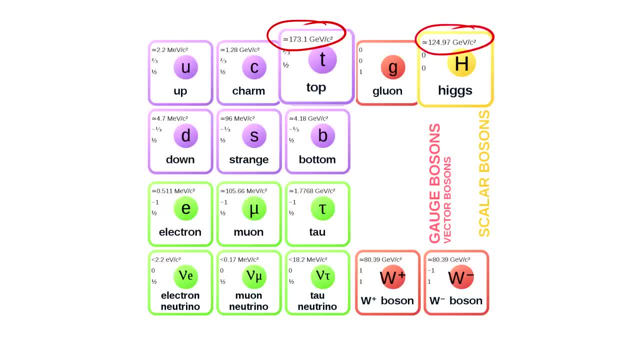 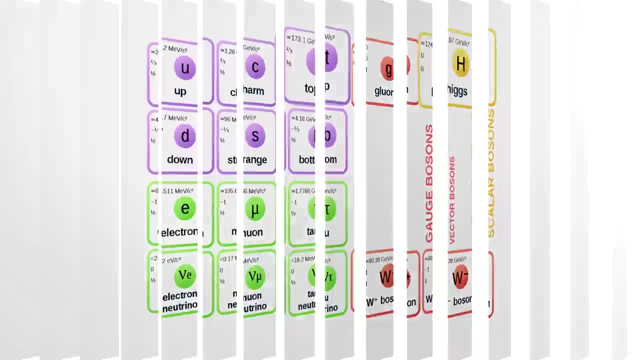 The top quark has the highest mass of all elementary particles, It has the best chance to decay into a Higgs boson. In general, when particles decay, they tend to decay into the next highest mass particle. Now, even though there are an endless number of Feynman diagrams, if you understood the